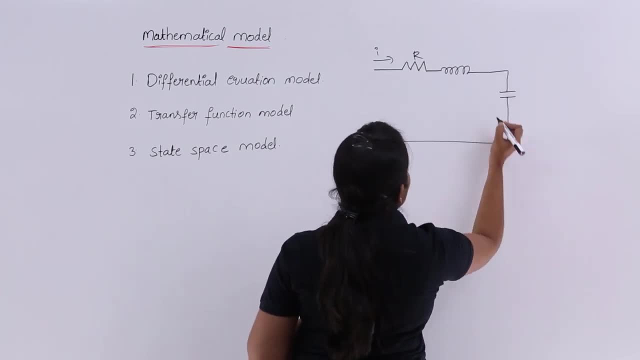 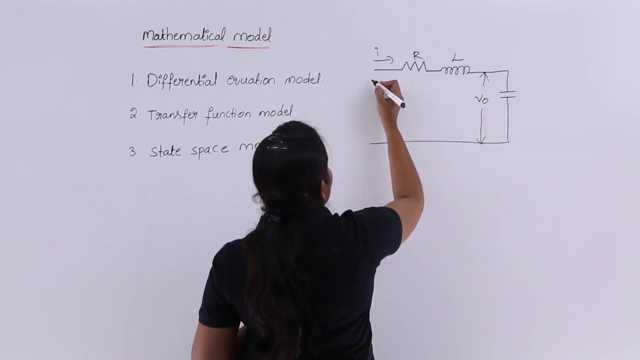 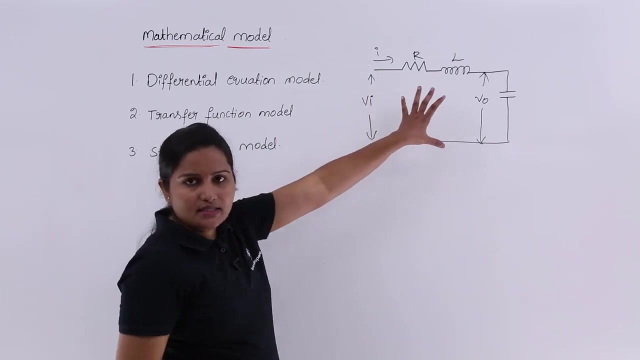 a capacitor C. So this is my system, this the output voltage across capacitor, and this is L, and here I am having VI. So here I am having input voltage VI. This is the system I am having. So now here. 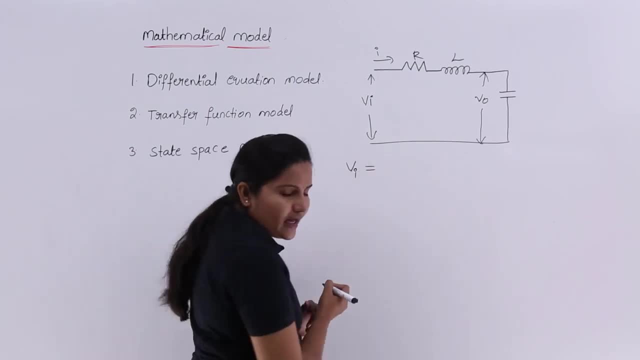 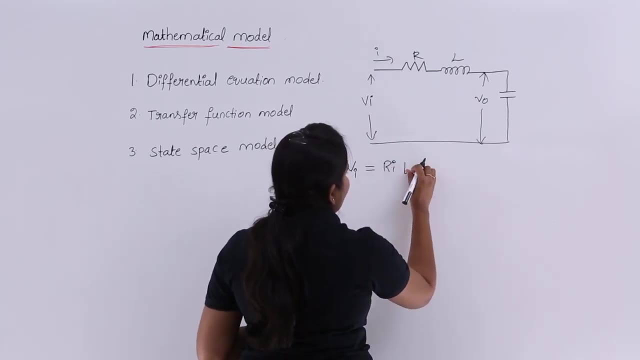 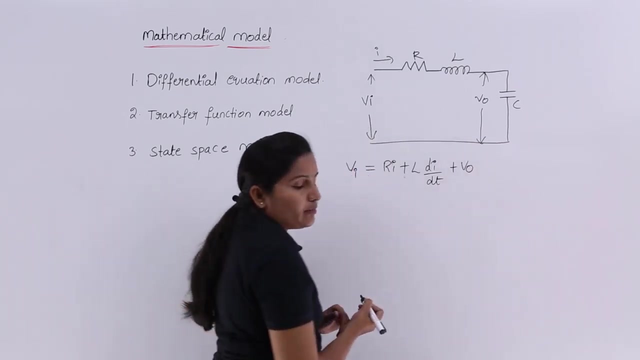 So here, if I want to write the equation for VI input voltage, this is equivalent to RI plus L into di by dt, plus voltage across inductor L into di by dt. Voltage across this capacitor is V naught. I am writing like V naught. So RI is the voltage across R voltage. 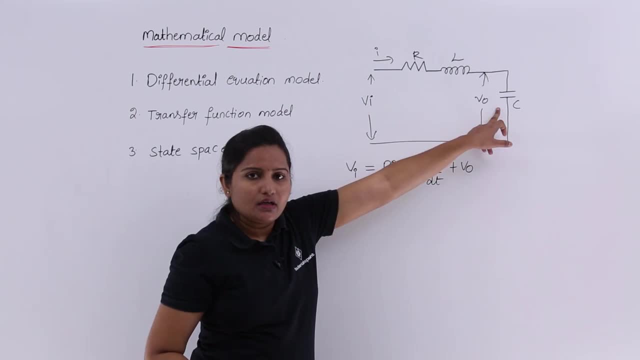 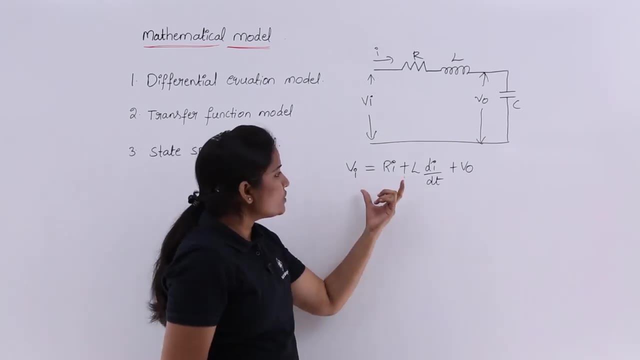 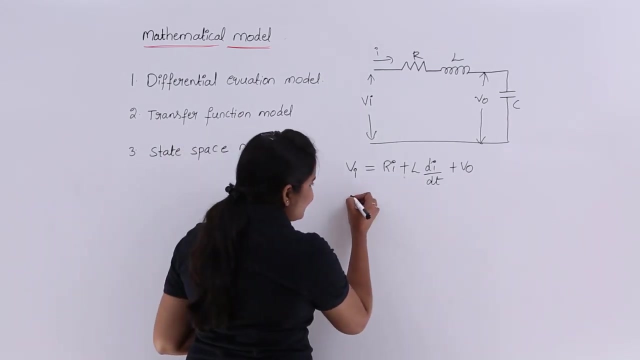 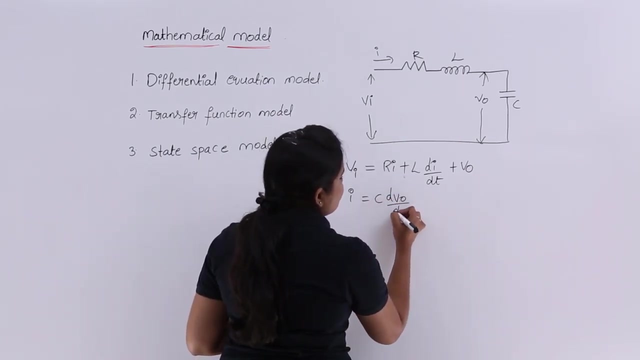 across inductor and voltage across this capacitor is equivalent to V. naught Why? Because in parallel voltage is equivalent to same, So here VI is equivalent to this one. So here I want to consider my current I in terms of capacitance as C into dV, naught by dt. So 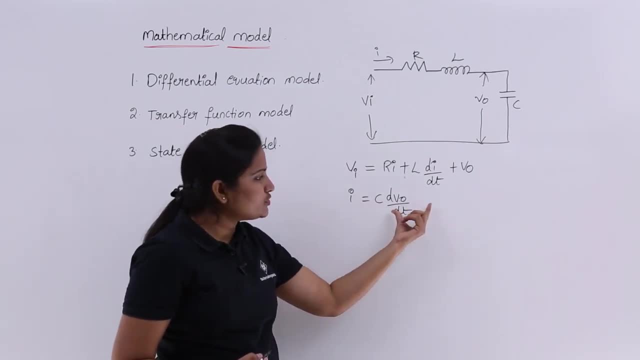 V naught is equal to C into dV naught by dt. so V naught is equal to. I is equivalent to C into dV naught by dt. I can write my I, in terms of capacitance, as C into dV naught by. 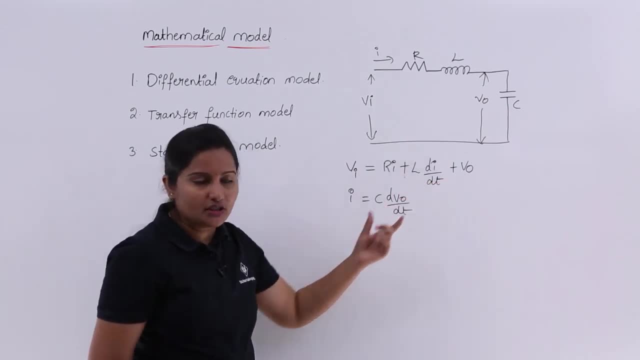 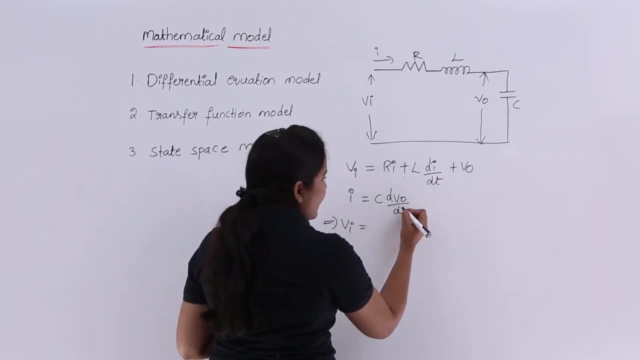 dt, which I can substitute in this equation. So then I am going to get my V I, as V I is equivalent to. in place of I, I can substitute R C into dV, naught by dt plus L C into So. 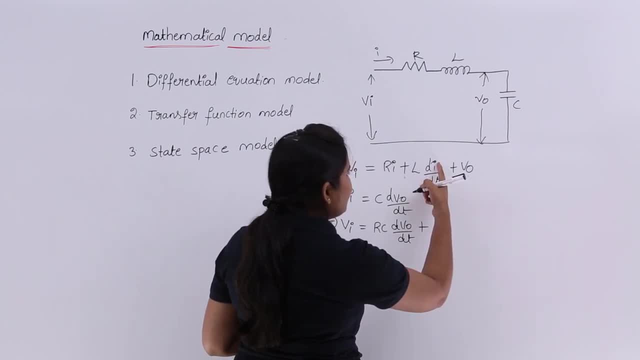 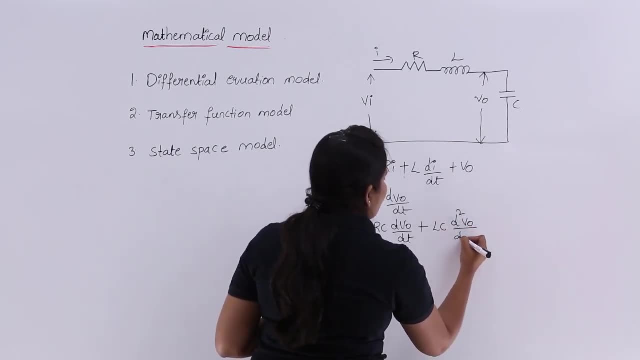 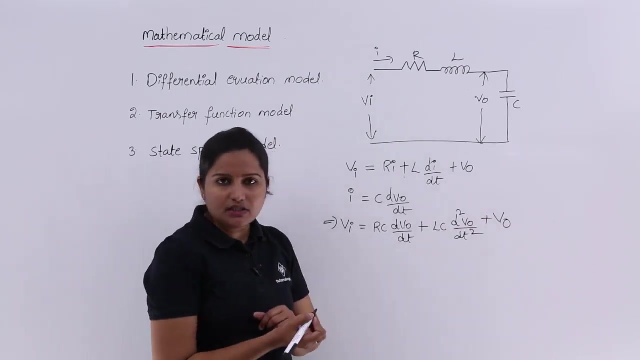 l c into. in place of i i can write c into d v naught by d t. that means d square, v naught by d t square plus. here i am having just v naught, so no need to substitute i. here i am not having any, i factor. that is why i am writing v naught, and here i want to take common of. 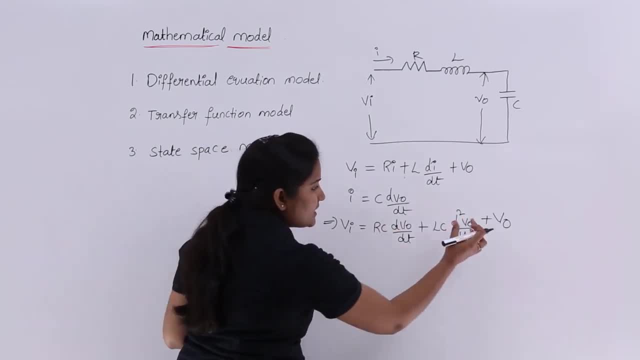 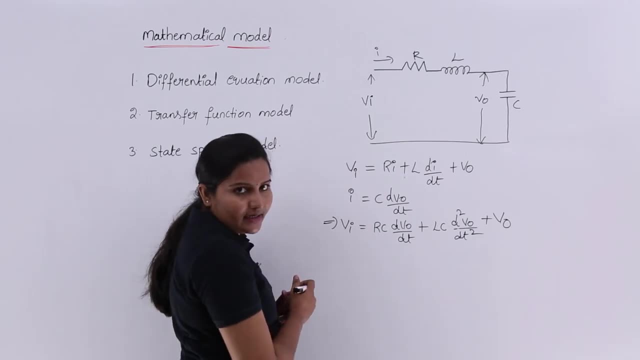 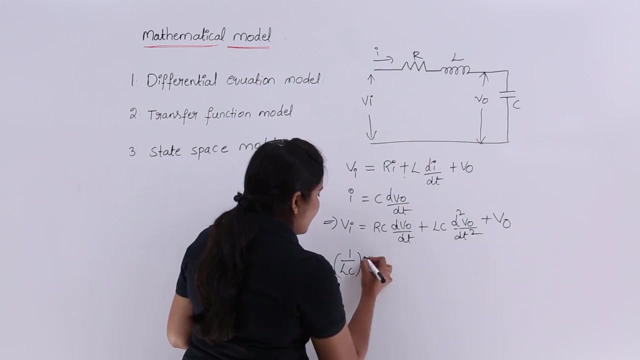 l c from here. so that means i want to consider my equation in terms of d square, v naught by d t square. i want to take common of this l c and i want to send this side. so here this is equivalent to one by l c into v. i is equivalent to r by l into d v naught by d t. so if i take common, then r c by l c will come. then i will get common of l c by v, naught by dt. that means blown out and that means that is maximum byedel feed the product for q t, sorry, what is the ratio of integration of these total sieves and so on. So that is a constant loss or conversion. 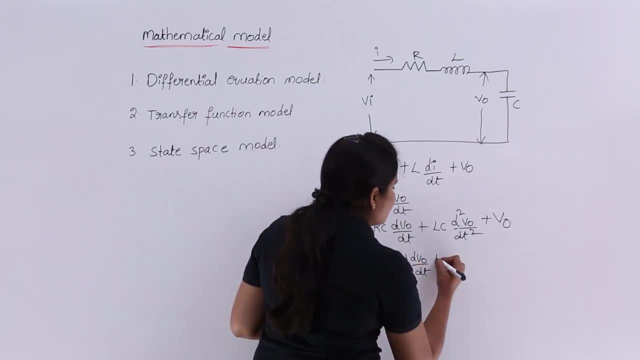 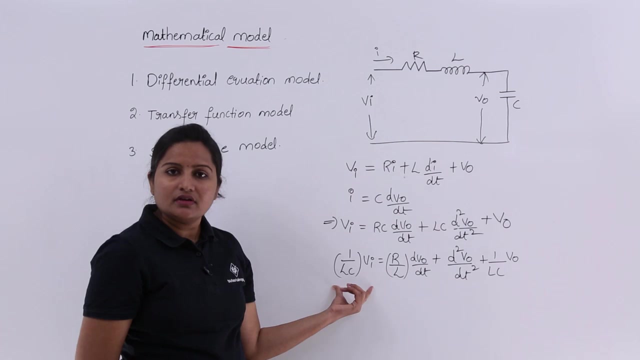 r by l into d v, naught by dt plus d square v, naught by dt square plus 1 by l c into v naught, I will get like this: So you can see, this equation is in terms of differential equation. So this equation, or this equation, is in terms of differential equation. So 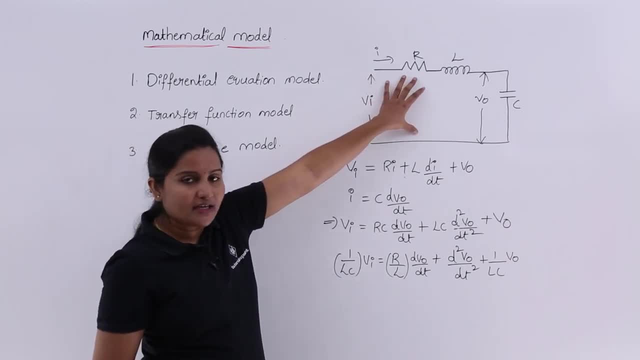 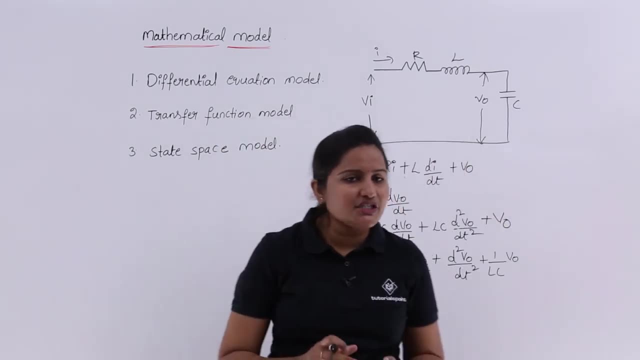 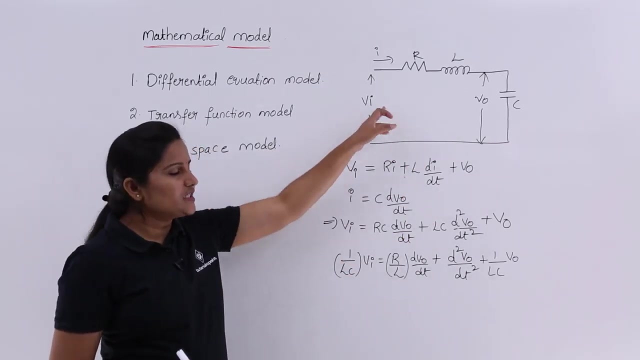 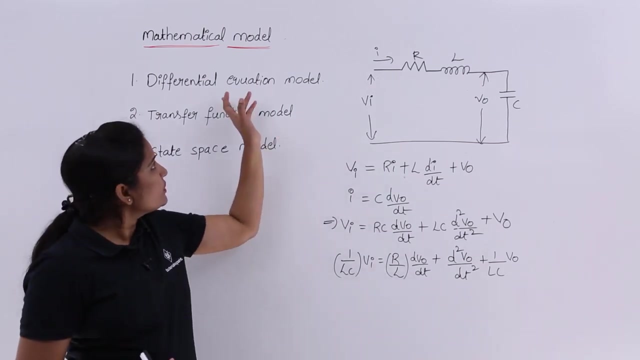 this equation generally describes the functionality of this circuit, So we can say this is called as differential equation model. what is the differential equation model of this circuit? means this equation? This is the differential equation model for this circuit. if they are asking what is the transfer function model? So to get the differential 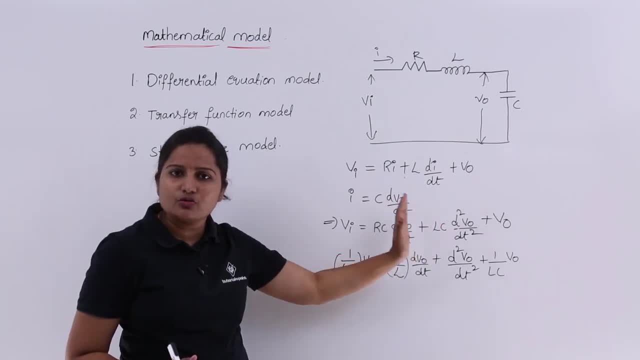 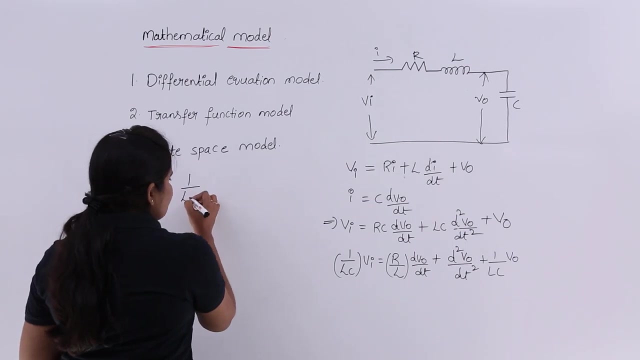 equation model. we need to just apply the general rules of this circuit circuit and after that we will get an equation. When you got that differential equation form, to get transfer function form you need to apply the Laplace transform here. So you can see: if you apply Laplace transform here, then you are going to get 1 by LC into. 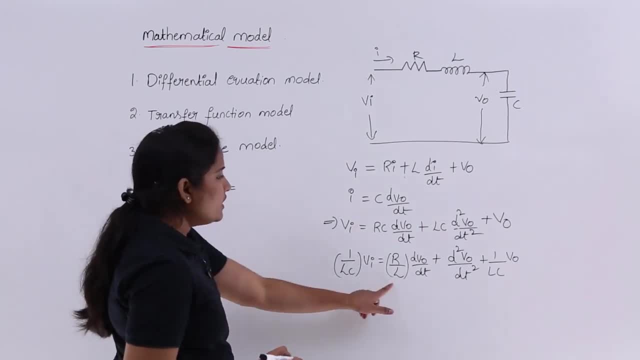 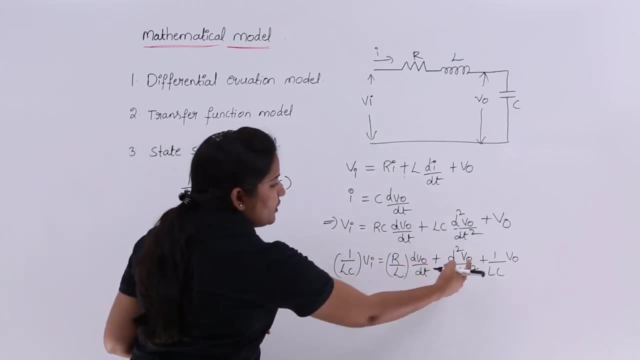 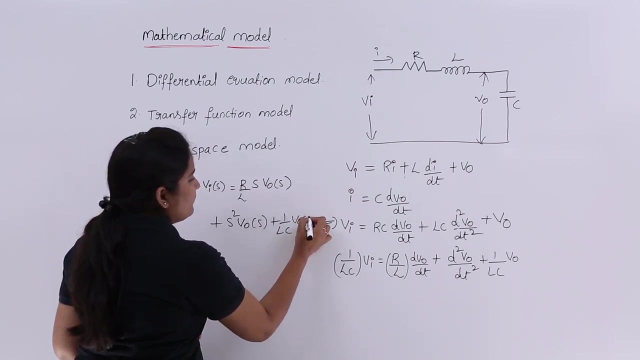 VI of S is equivalent to R by L into S, into V naught of S plus d square, V naught by dt square. that means S square into V naught of S, plus 1 by LC into V naught of S. So this side I am taking common of this V naught of S. So 1 by LC into VI of S is.